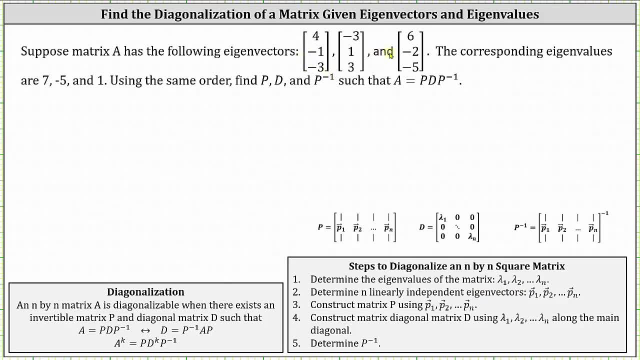 which again has already been done for us. Those are the three given eigenvectors. And then we construct matrix P using the eigenvectors and then construct the diagonal matrix D using the eigenvectors. So we have three values along the main diagonal. 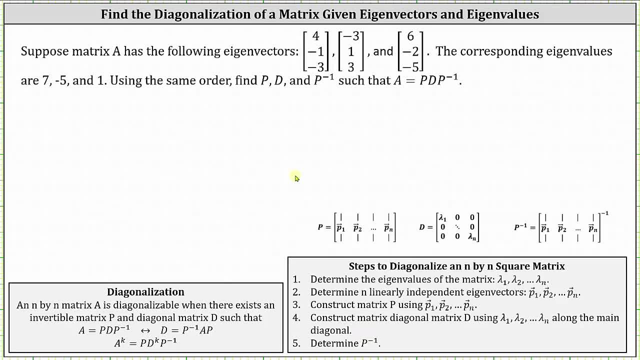 And then the final step, which we still have to do, is to determine P inverse. So, again from the given information, we know that matrix P is formed using the given eigenvectors, where the first column is four negative one, negative three. 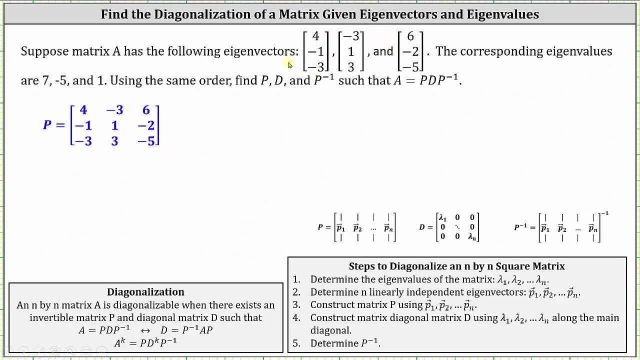 The second column is negative three, one, three And the third column is six negative, two negative five. We also know the diagonal matrix D has the entries of seven negative five, one along the main diagonal. It is important to make sure. 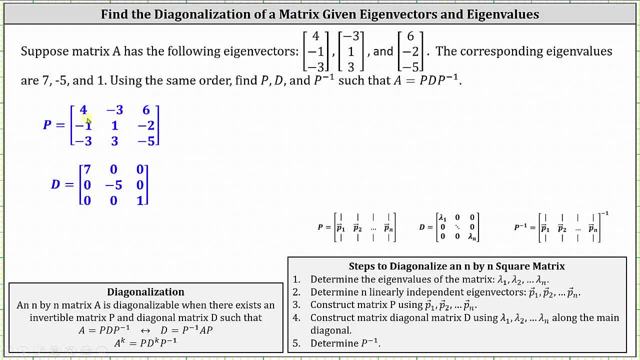 that the corresponding columns do contain the eigenvector and the corresponding eigenvalue. For example, the eigenvector of four negative one- negative three corresponds to the eigenvalue of seven. The eigenvector of negative one one three corresponds to the eigenvalue of negative five. 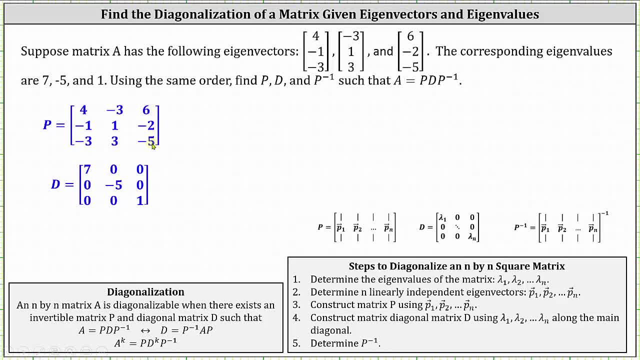 And the eigenvector six negative, two negative five corresponds to the eigenvalue of positive one. To complete the diagonalization of matrix A, we need to find the inverse of matrix P. There's a couple of ways we can do this. 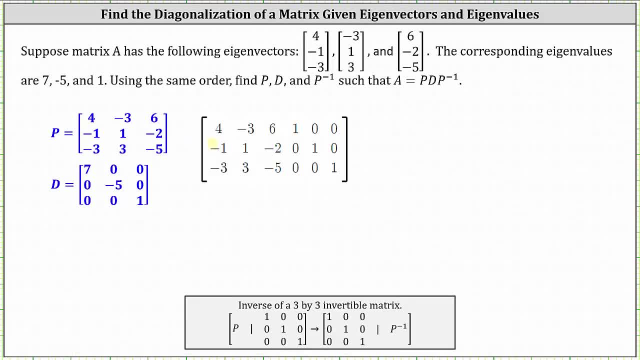 I'm going to go ahead and use an augmented matrix where, if we set this up so that the first three columns are matrix P and then columns four, five and six are the identity matrix, we can then perform raw operations so that we have the identity matrix on the left. 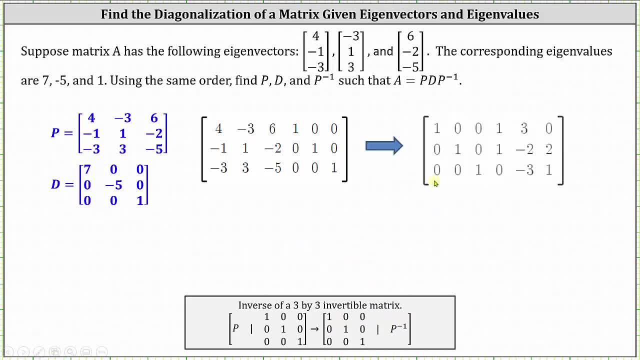 and the entries on the right will be P inverse. So I've already done all the row operations and this is our result. Notice how we have the three by three identity matrix on the left, The inverse of matrix P. matrix P is on the right. 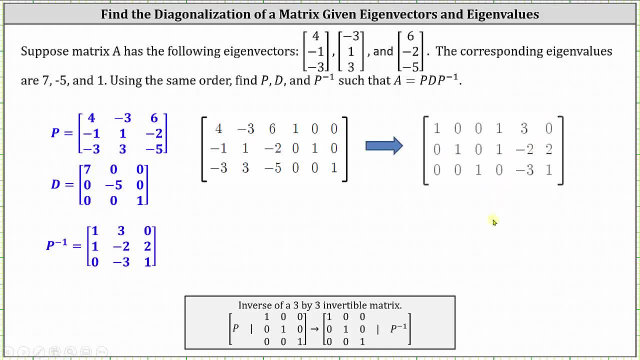 The inverse of matrix P is the three by three matrix where the entries are one, three, zero, one negative two, two and zero negative three, one, which is listed here at the bottom. So now we know the diagonalization of matrix A. 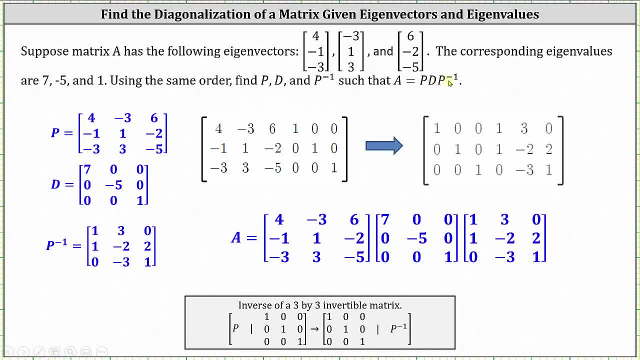 is equal to, again, P times D times P inverse, where, again, matrix P is formed using the eigenvectors, matrix D is formed using the eigenvalues, and the third matrix is the inverse of matrix P. So this is what the question is asking us to find. 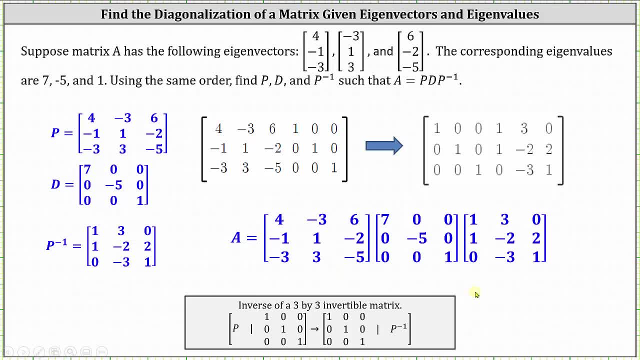 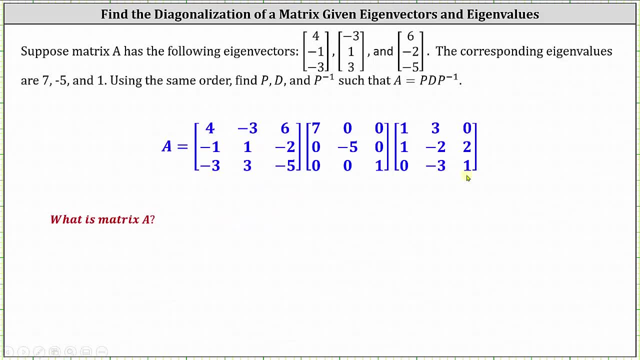 If we did want to find matrix A, we would have to determine the product of these three matrices, which I thought would be worth showing If you pause the video and multiply these matrices out from left to right. matrix A is the matrix with entries 43,, 36,, 36, negative 12,. 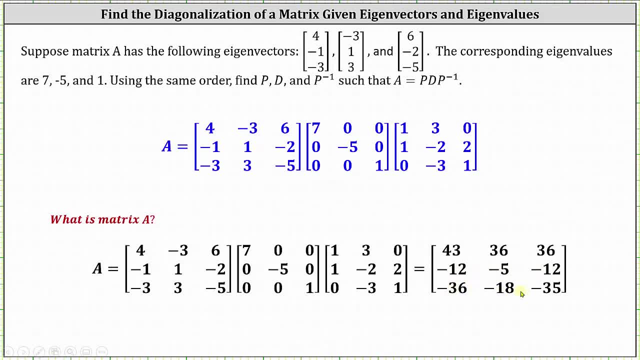 negative five negative 12, negative 36, negative 18, negative 35.. I hope you found this helpful. 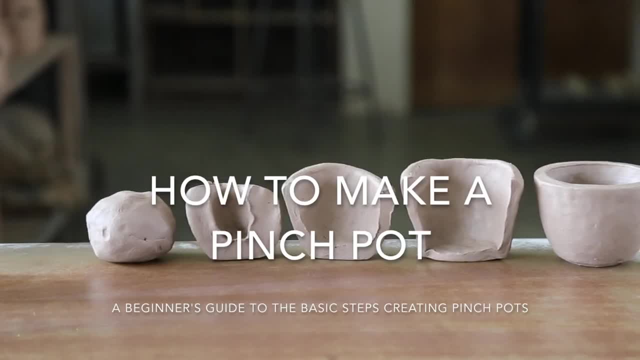 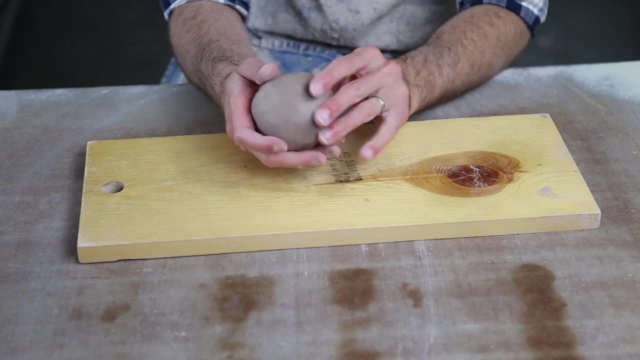 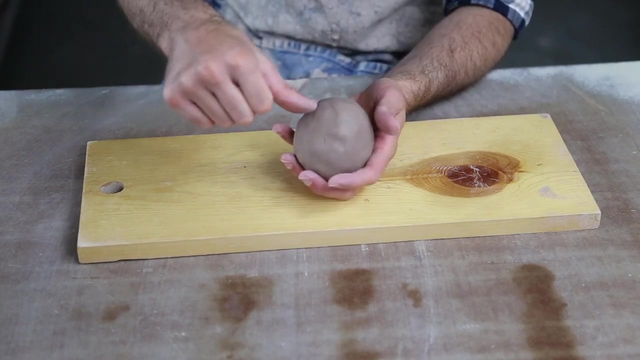 Hey folks, today I'm going to teach you how to make a pinch pot. By now you should have already wedged out a one pound chunk of clay. Now you're going to slap and wad it into a perfectly round ball. Next take your thumb and puncture down into the ball of clay. 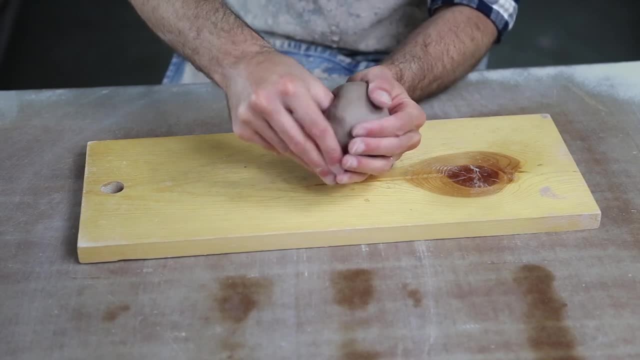 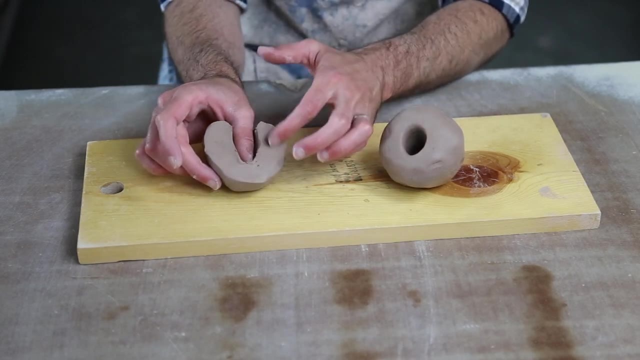 but be careful not to perforate the base. You're going to need that. If we look at the inside profile, this is what you would see As I pinch the clay from the bottom to the top and top to bottom. it's going to eventually thin out. 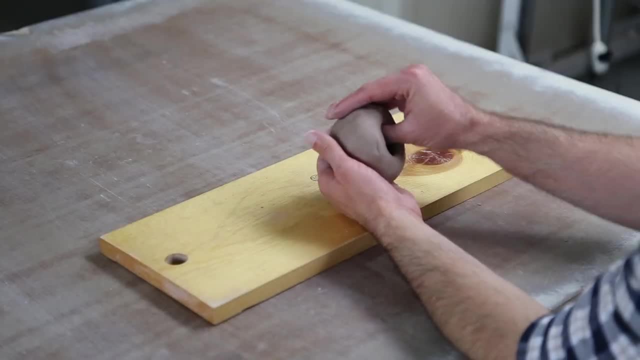 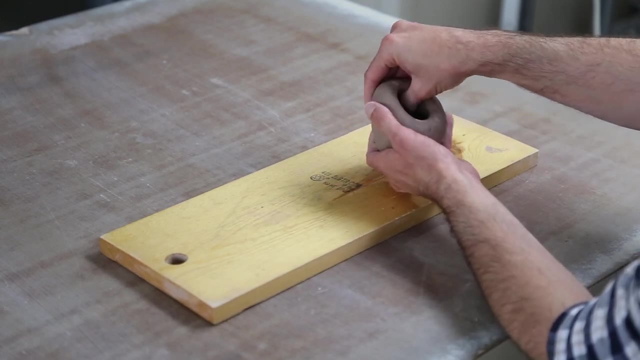 As I pinch around the inside with one hand, the mouth will get wider and I'll be able to fit two thumbs on the inside. As I apply pinching pressure from top to bottom and bottom to top, the pot will expand and eventually become thinner. I want you to notice how I'm using the table surface to support the side profile of the. 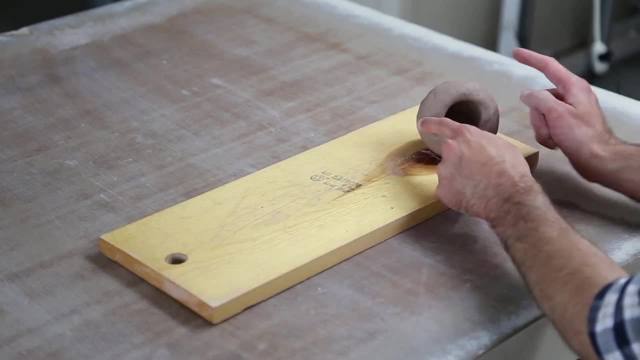 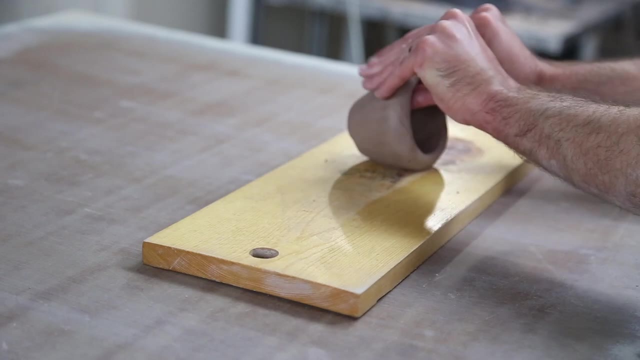 pinch pot. This allows me to keep it sturdy as I pinch and prevents it from flaring out too wide. Bending wheel would be preferable here, but it's likely that not everyone will be able to use one at the same time, so this is an easy accommodation. This is the basic pinching motion that I'm using.